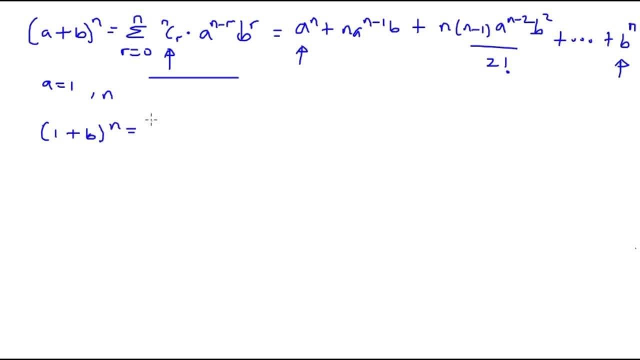 1 plus b raised to power n, and that's equal to 1 plus n, b plus n into n minus 1, then b squared upon 2 factorial plus okay, plus n into n minus 1, n minus 2, b cubed upon 3 factorial plus dot, dot dot. 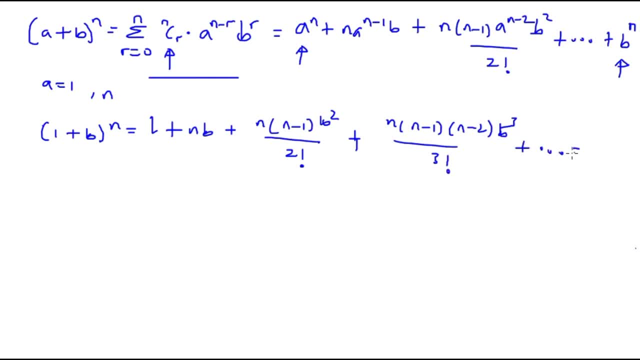 so it continues like that. okay, to the point where i will have n summation r equal to 0, then 1 is still the same thing. i won't have 1, i will just have n combination r. i don't need to have 1 raised to power n minus r, because 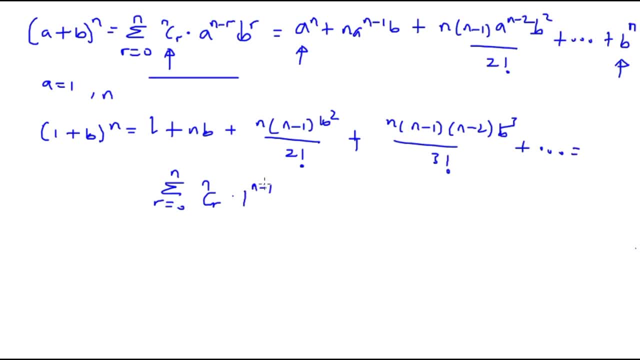 1 raised to power n minus r is still the same thing as 1. okay, so i don't need to write that. so i just need to write: go straight to b raised to power r. okay, so that is what the expansion will yield. okay, but notice that. 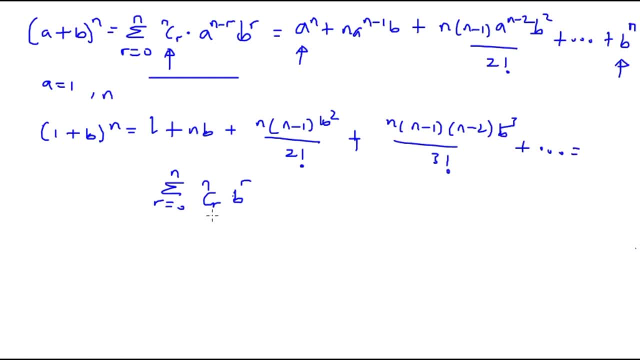 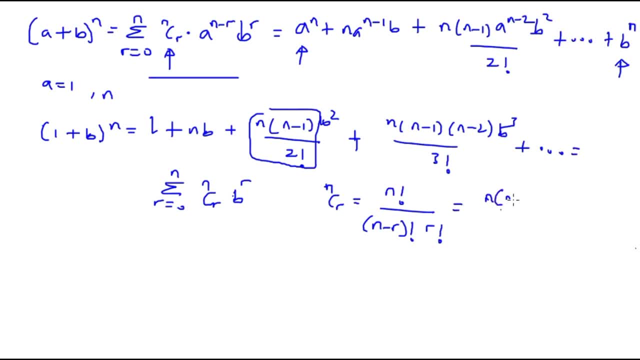 so, so, so, for so, so, and we so, so, and we so so: n minus 1 to a point where we have n minus r plus 1. okay, and then upon r factorial, where r will be increasing from 0 to a point where you will get. 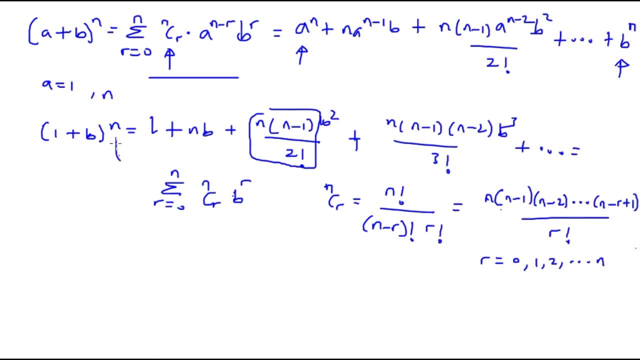 to n. n is the maximum number, n is the maximum number, so this formula works for all kinds of binomial. okay, so let's say we want to use this formula to solve this binomial expansion 2x minus 3 raised to power 4. okay, normally you can. you can do this directly with this. 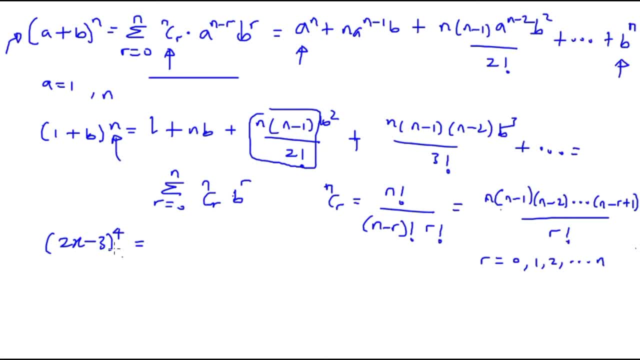 formula right here. okay, you can expand it directly without formula, but we want to use this approach so we can see. so the first thing, if you want to use that approach it's to is to find a way to to fact is to find a way to change the form. 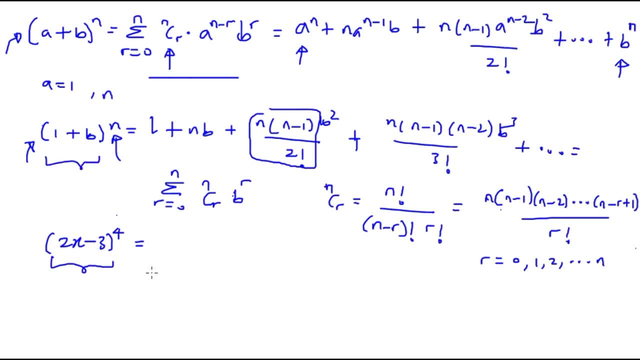 of this binomial to this form. and for us to do that we need to factorize minus 3 out of the binomial so that if we factorize minus 3 out of the binomial, will be able to have one right here and then the other parts of the binomial. 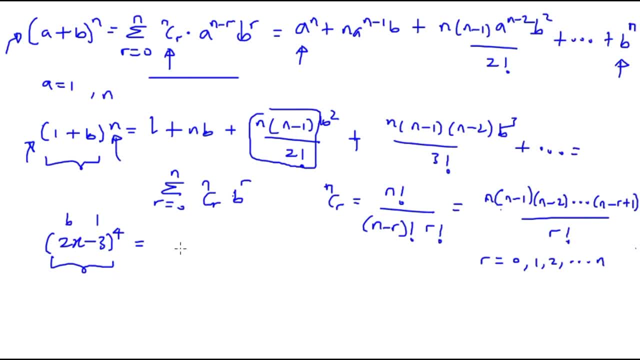 will be our B. okay. so if I factorize minus 3 out of the binomial, I should have 2x upon minus 3 plus 1. okay, since I already took out minus 3, then the thing that will be left there is plus 1. okay, so you can try to expand the bracket. you still have 2x. 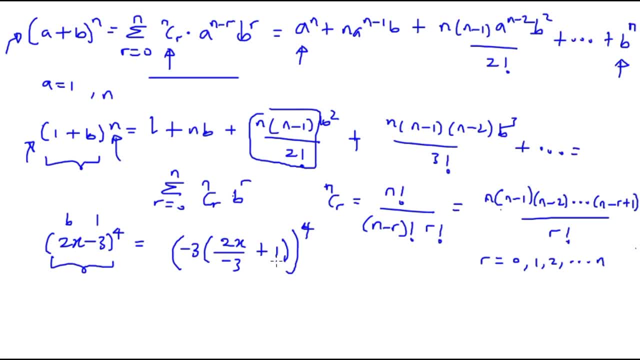 minus 3. so that's how to do it. whatever you take out of here, you put it as the denominator of the other side of the binomial, so we can split the binomial, so that we can have minus 3 raised to power 4 and then properly we 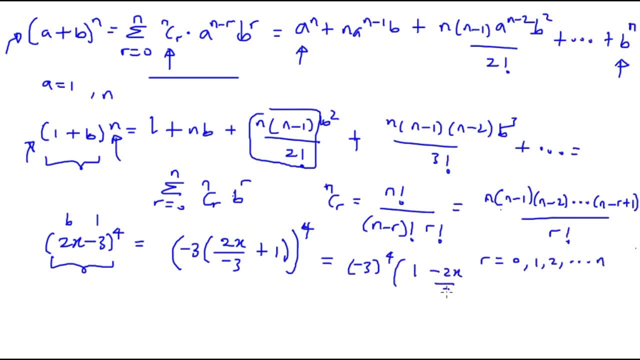 can write: 1 minus 2x upon 3 raised to power 4: okay. so if you decide to expand this binomial, 1 minus 2x upon 3 raised to power 4, okay, if you expand it, you will have the term. you have a. 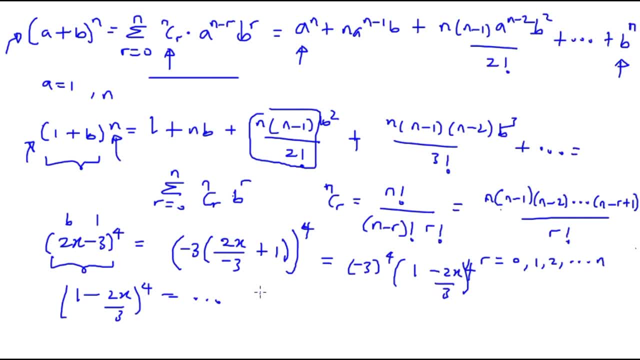 particular binomial which will be valid if the absolute value of X. okay, I forgot to say that this formula is only valid when the absolute value of whatever you have at the point at this part of at this B part, when the absolute values is less than one. 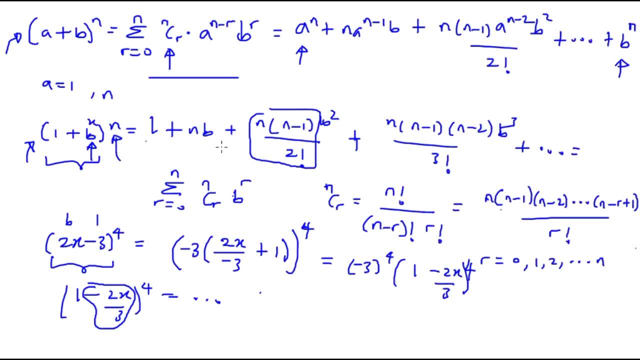 let's say you have X at this part. so this formula will be valid only when the absolute value of X is less than 1. but for this binomial that we have just expanded, it will only be valid if minus 2x upon theory is less than 1. so if whenever? 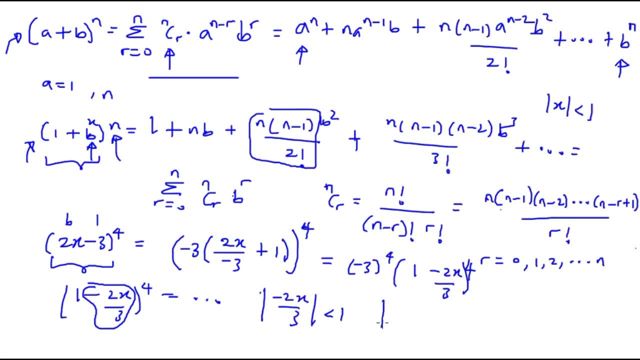 you are using absolute value, you don't need to make use of the sign. so we can say that you don't need to make use of the sign and the constant value. so we can bring out 2 upon 3 and then we can say that X- absolute value of X- is less. 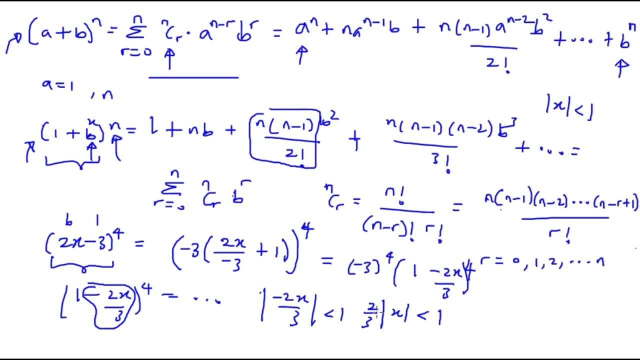 than 1. so the sign is: whenever we are making use of absolute value, we don't consider sign okay, whether positive or negative, we don't consider. so if I multiply through this inequality right here by 3 over 2, the inequality will be balanced, and then now we have 3 over 2 at the other side, so it is only valid. 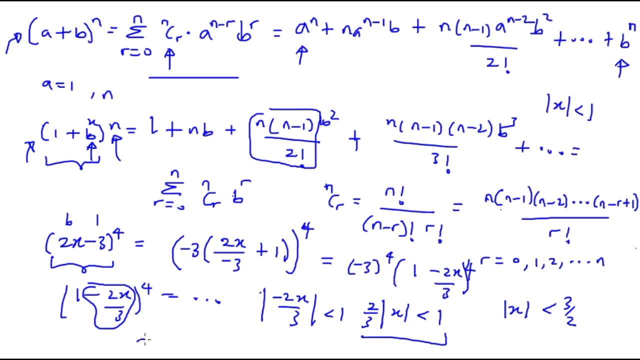 now, after you have expanded this, you just need to make use of this binomial and then you can say that you don't need to multiply with minus 3 raised to power 4. minus 3 raised to power 4 is 81, so 81. 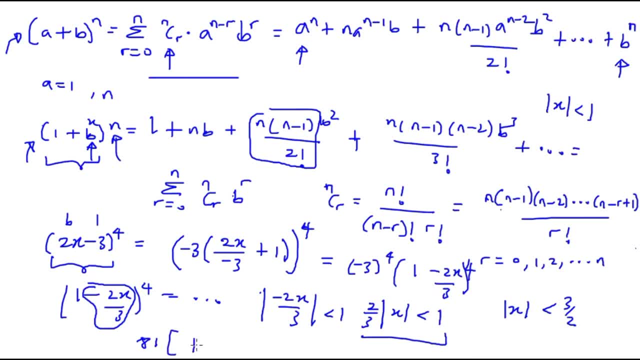 multiplied by this expansion, 1 minus 2x upon 3, raised to power 4, if you do it correctly, you will have the same expansion that you have if you are done it directly with this first formula that we use when we were considering binomial. 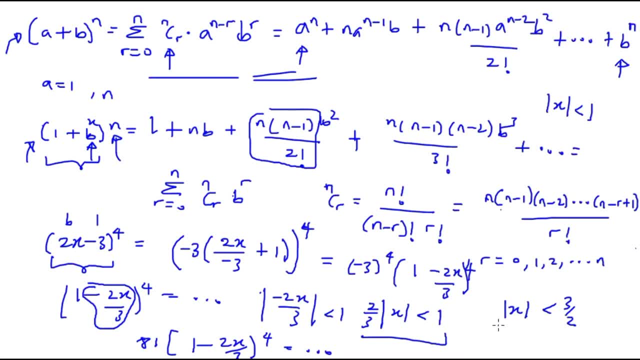 expansion for positive integer. the only thing that is different is that if you use this formula of one plus, you will be constrained with this condition. okay, so it is better, whenever you have positive power to use, to expand directly. now let's go straight to binomial. let's go straight to examples with negative powers. so recall that the 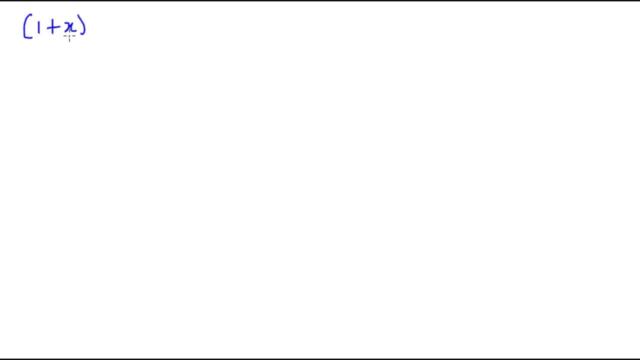 formula is 1 plus X, so we can have B, we can have X, anything raised to power minus minus n. okay, now n is negative. okay, so we can say that this is 1 minus nx. okay, actually we're supposed to have 1 plus nx, but since n is now negative, so that's what we have. okay, plus instead. 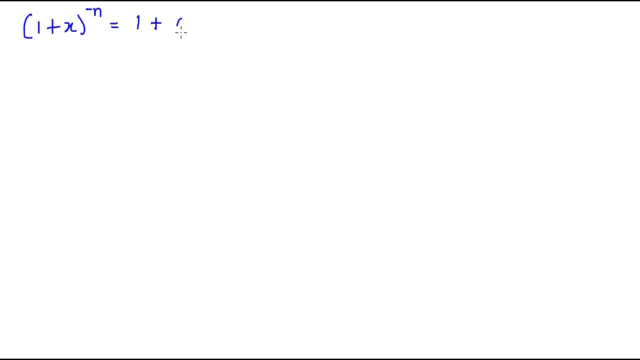 instead of doing it that way, i can see 1 plus minus nx- okay, plus minus n into minus n minus 1, minus okay, minus n minus 1, and then i'll have x squared upon 2 factorial plus minus n into minus n minus 1, okay, and then. 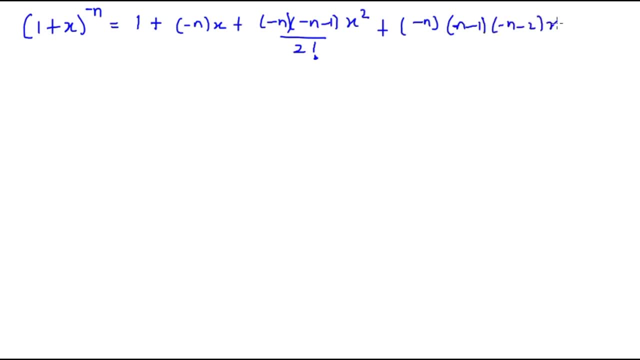 minus n minus 2. okay, x cube upon 3 factorial. so i'll continue to have the formula. it will not come to an end. the formula will not come to an end, unlike when we have positive n. if i have positive n, i will get to a point where i will say n minus r and that n minus r will be equal to 0. 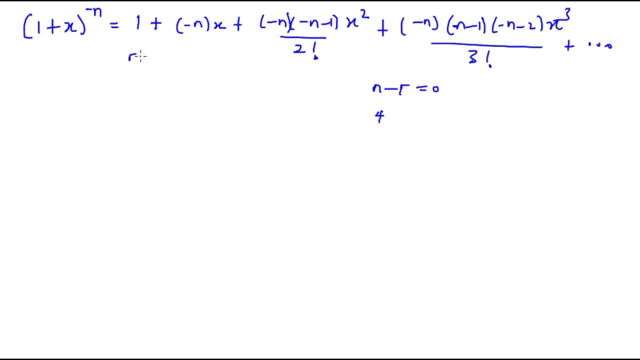 it will be equal to 0. this is the point where i is equal to 0. this is r equal to 1. this is r equal to 2. this is r equal to 3. let's say i have a binomial expansion where n is 2. okay, let's say i have 1 plus x raised to power 2. i will 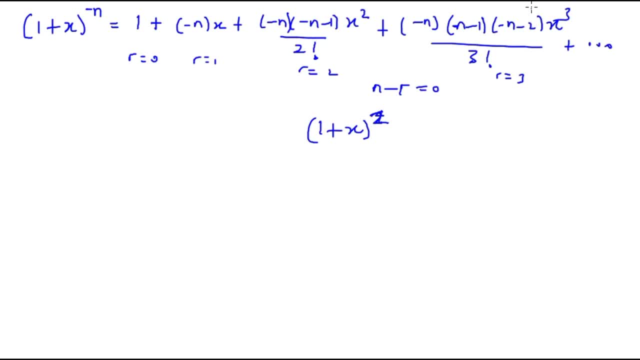 do it to a point where i will say n minus 2, that means this place will be equal to 0. that means i will not have this term. okay, so it will terminate at this time. and that's why positive power binomials are not, is not, is is not an infinite series. it's a finite series because 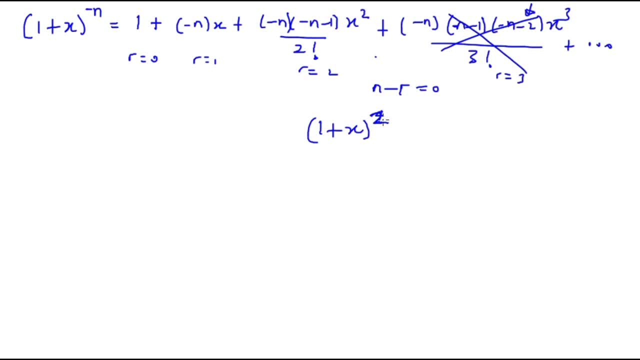 it should terminate at a particular point. but negative integer binomial is an infinite series. so if i have minus 2 at this point, it will be minus 2, minus 2, which is still minus 4 and is not 0, so it does not terminate. so negative power binomial are infinite series, while positive power. 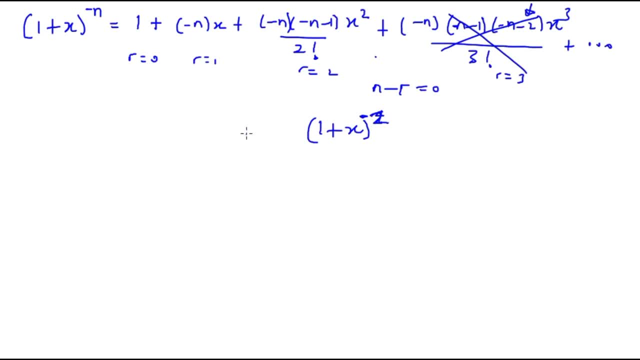 power binomial is a finite series, while negative power binomial is an infinite series. now let's continue with the solution. another thing that is crucial is that you need to know this formula at art, like from: from this point: from this point, you just need to say that 1 plus 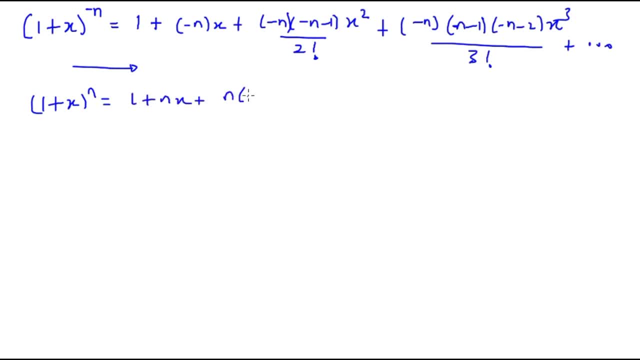 n, x plus n will be in a factorial form: n minus 1, then x squared upon 2 factorial. whatever you have right here is what you have right here, and it continues like that. okay, so you just need to know that. now let's solve an example. so let's say you want to expand. 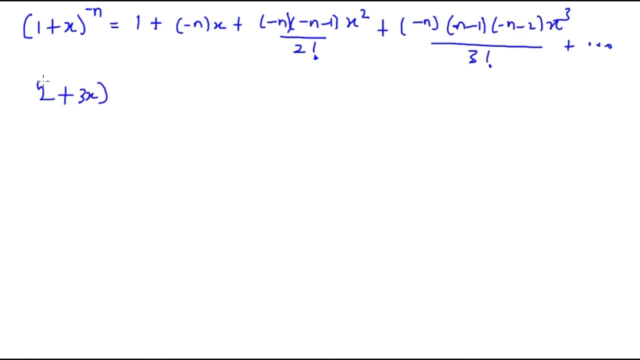 2 plus 3x raised to power minus 6. okay, 2 plus 3x is to power minus, so the the first thing i will do is to let it be in this form. okay, that means, don't forget that this formula is only valid, okay, if whatever we have here, that is. 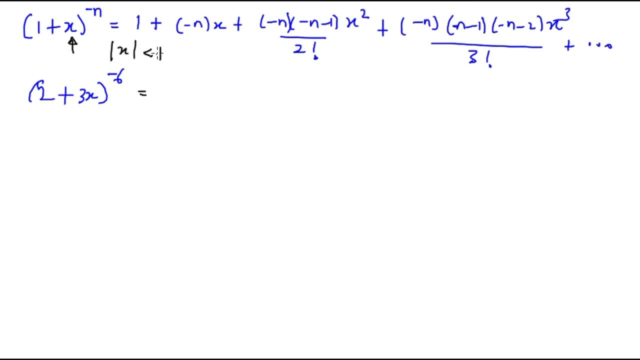 the absolute value of x is less than one. that's the only condition. okay, it's the binomix. the formula is valid for all kinds of binomial, but it has a condition now. so for me to continue, i just need to put this binomial in its form, that general form. so that means i need to bring out: 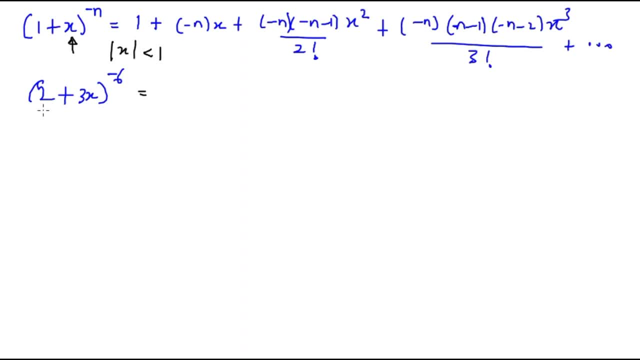 x by the square root of minus 2, so that if i bring out by the method of factorization i'll be able to have one right. so if i bring out, if i factorize 2, if i have 1 plus 3x upon 2, 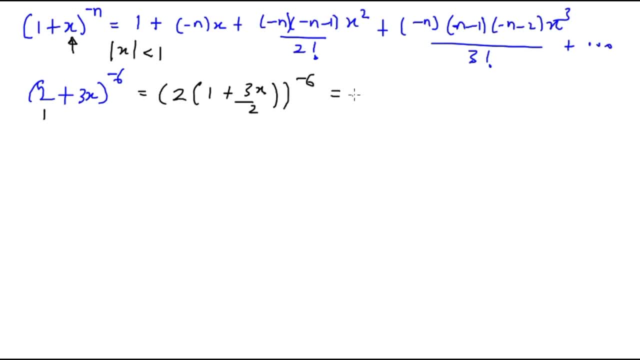 and then i'll have everything under minus 6 as a power. so it's the same thing as 2 raised to power minus 6 into 1 plus 3x upon 2, then raise to the power minus 6, 6. okay, so I just need to expand 1 plus 3x upon 2 with binomial expansion, okay. 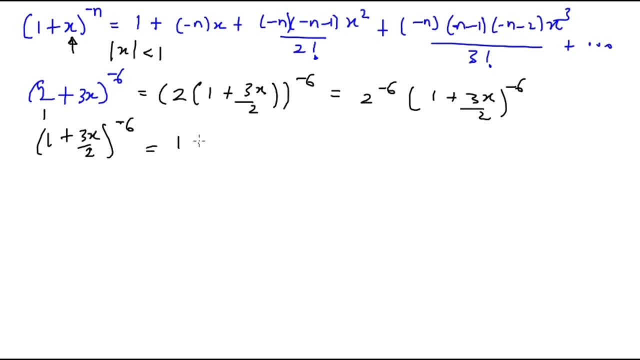 and I'll have 1 plus minus 6, then X isn't it, and X will be replaced by 3x upon 2 plus minus 6. again, then I need to say minus 6 minus 1, and that is minus 7. and that's upon what? 2 factorial, and that's what 3x over 2 squared, isn't it? 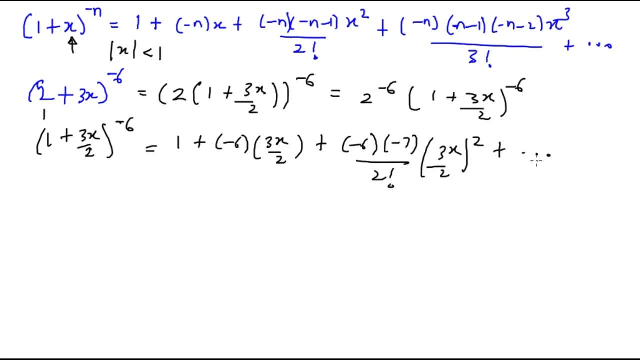 so it's an infinite series. I don't need to continue because our is infinite, so I just need to stop somewhere. okay, so eventually I'll have 1 minus 9x. okay, that should be 9 plus. you know, this is 2 factorial. 2 factorial means 2 times 1. okay, so if I minus and minus, that's positive, so 2. 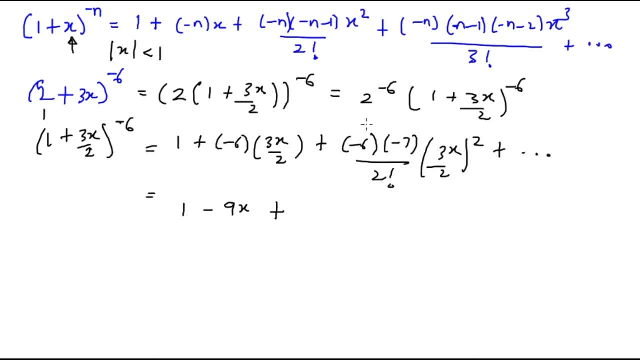 factorial. it should cancel out 3 to give us. it should cancel out 6 to give us 6 to give us 3. okay, so I should have 7 times 3, which is 21. so that's actually 189, 189 X squared over 2. so 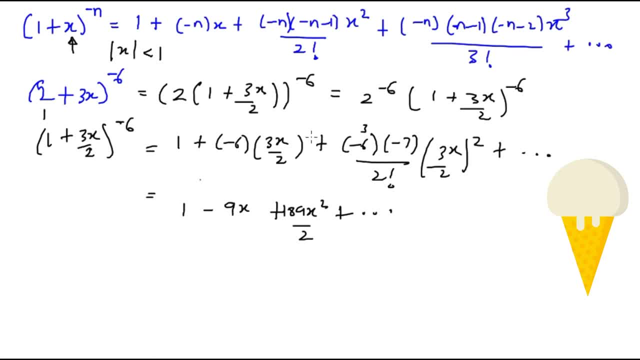 plus dot, dot dot. okay, so that is the binomial. so I just need to multiply the binomial. but 2 raised to power minus 6. don't forget that 2 raised to power minus 6 is actually 1 over 64, because 2 raised to power minus 6 is the same thing as 1. 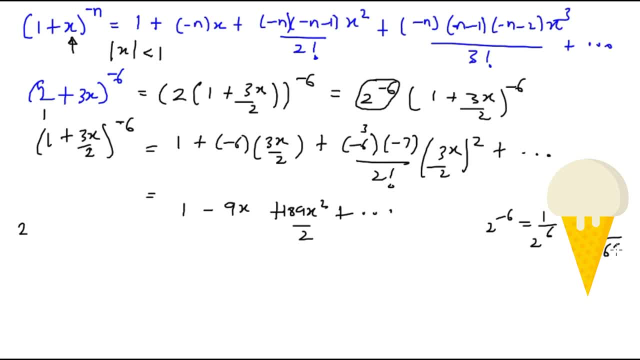 over 2, raised to power 6, and that's 1 over 64. so I will eventually have 1 over 64 to multiply: 1 minus 9x plus 189 X. squared upon 2 plus dot dot dot is an infinite series. so my final. 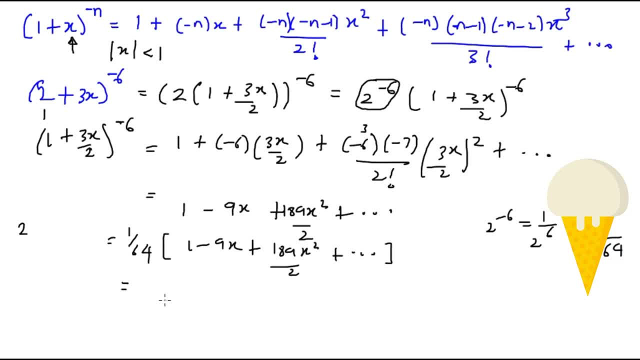 answer will be attracted to distribute one over 64 throughout, so that our we have one over 64 minus 9, X upon 64 plus that should be one. it's 189 over four, x by 1 over 64. at least something should be reduced to our 189 over 256, 189 upon. 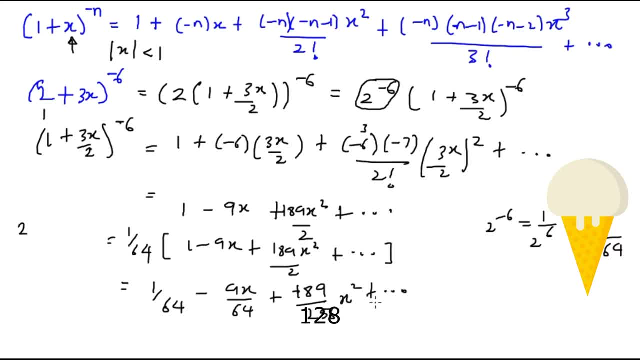 x squared plus dot dot dot. so that is the binomial and it is only valid if- check this place- if 3x upon 2, if the absolute value of 3x upon 2 is less than 1. so we bring out every other thing. 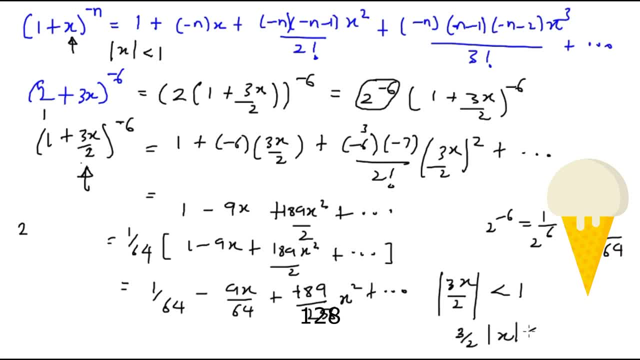 that's 3 upon 2. absolute value of x less than 1. if i multiply through the binomial by 3 over 2, i should have absolute value of x less than 2 over 3. so i need to multiply both sides by 2 over 3 just to balance. 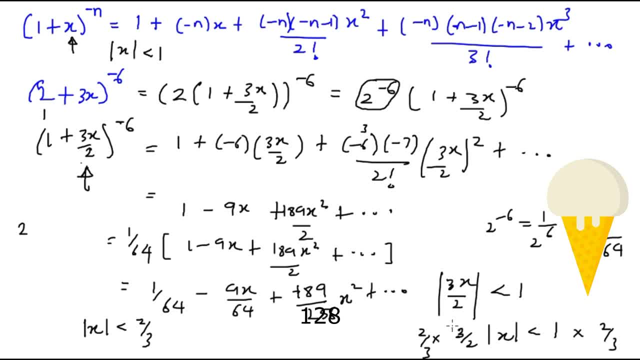 to balance the inequality so that today will cancel out from this place and then i'll have this. so it's as simple as that. if you don't understand what this actually means in the real sense, you can watch my video where i, where i already treated everything about. 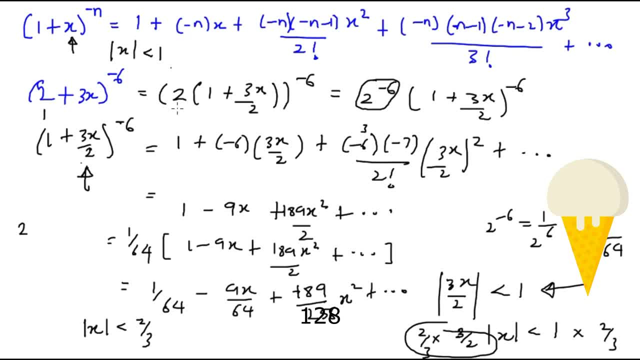 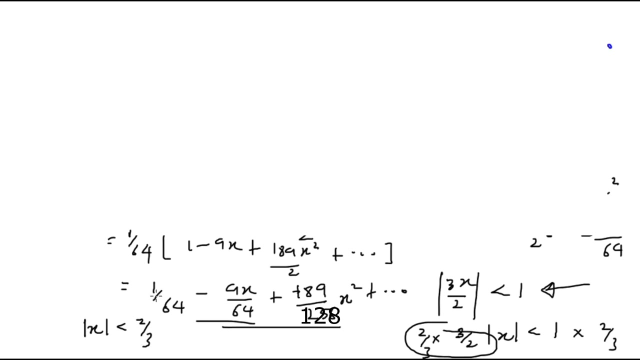 absolute value: inequality. now, we can test this binomial if it is correct. this is the answer. but we can test it. if it is correct, okay to test it. we have said that. we have said that the binomial is valid. okay, is valid only when we have said that the binomial is valid when the absolute value of x is less. 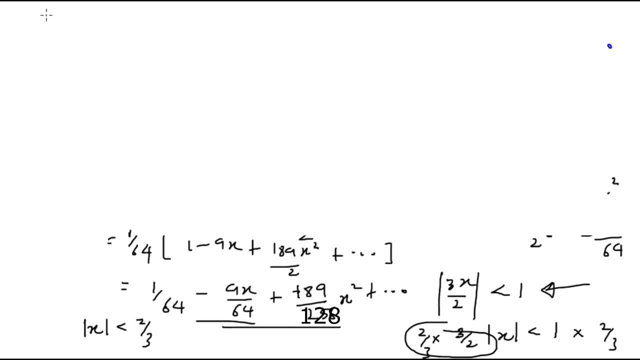 than 2 over 3, and what that actually means is that x is less than 2 over 3 and x is greater than minus 2 over 3. okay, so 2 over 3 is actually 0.67. so i have something of this nature: 0.67, that's minus two over three. 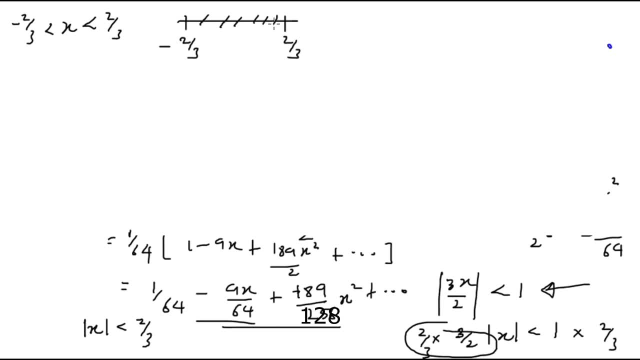 and then two over three. so the answers, the divide, the particular values of x actually lie in this middle, so it is between this region. okay, so if we pick a value in this region for us to take now, let's say we pick a value in this region. no, don't forget that the binomial that we expanded 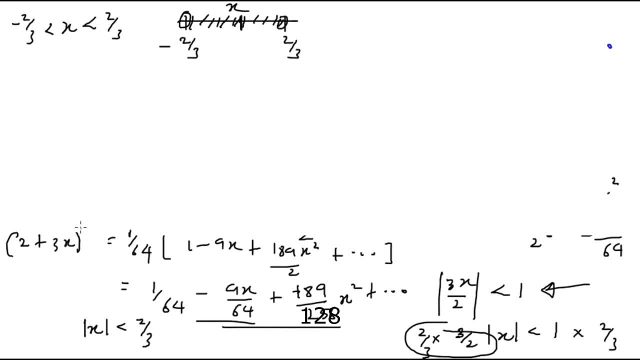 is actually 2 plus 3x, raised to power minus 6, and is equal to this. if it is equal to this, then we should. it should be correct. so if i pick a value in this region, let's say i pick up 0 as a value, if i substitute 0 in the left hand side, i will have 2, 3 times 0.0. that's 2 plus 0. 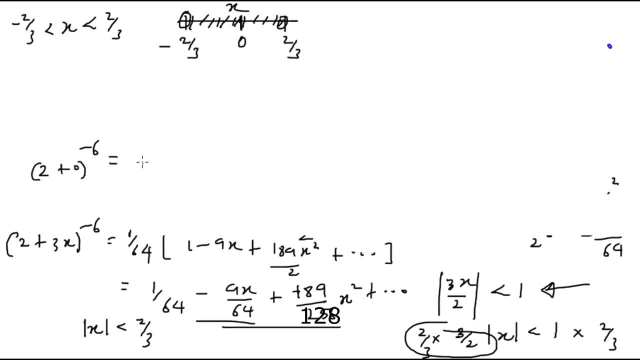 raised to power minus 6 and on the right hand side that we have 1 over 64 minus 9x is now zero. okay, we are testing out zero every other thing. if i plug zero on every other thing, it will become zero. so eventually my answer will be 1 over 64 for the right hand side. right, okay, don't let me. 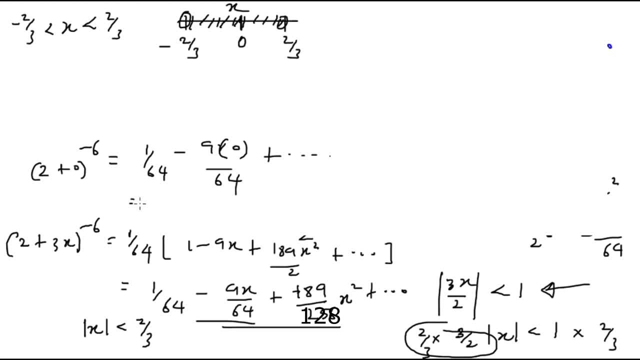 write it there. so for the right hand side, that we have 1 over 64, because 0 times all of this will be zero, zero other term as x, so it will be 0, and then 2 raised to power minus 6 is also 1 over 64, so it is valid. 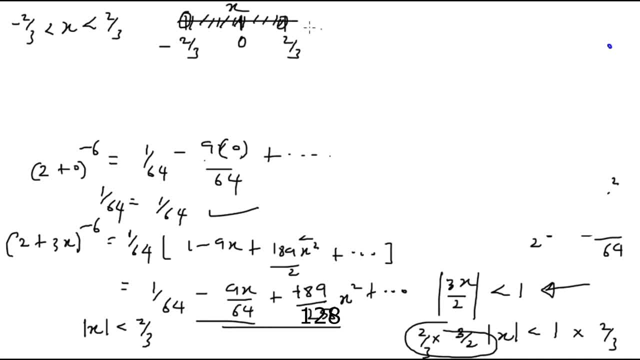 okay. but if i pick a number outside the region- let's say i pick up 5, which is not in the region- if i substitute 5, or let's say, let me just pick a number that is not too far like 1, if i pick up 1, 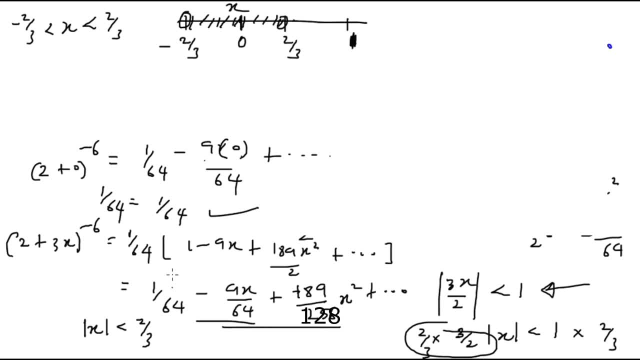 which is not in the region. if i pick up 1 and then i substitute okay, i'll have 2 plus 3 into 1, all raised to power minus 6, and that will be equal to 1 over 64 minus 9 upon 64. i have 1 right here. 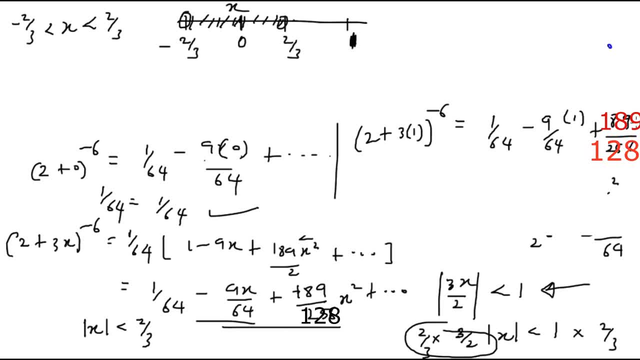 plus x squared, that's one square, so i don't need to include that. so at least it should be an approximating value. if, even if it's not equal to, should be an approximate value, because it's an infinite series. it does not terminate. so let's say: 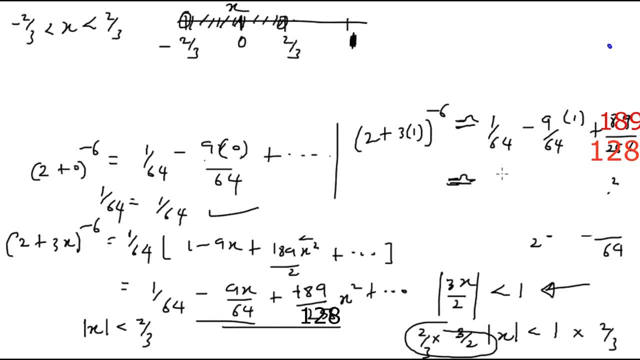 let's just calculate 1 upon 64 minus 9 upon 64, and then plus, and then 2 plus 3 raised to power minus 6, 2 plus 3, that's 5. so i have 5 raised to power minus 6.. 5 raised to power minus 6 is is 6.4 exponential minus 5, so they are not approximate values at all. 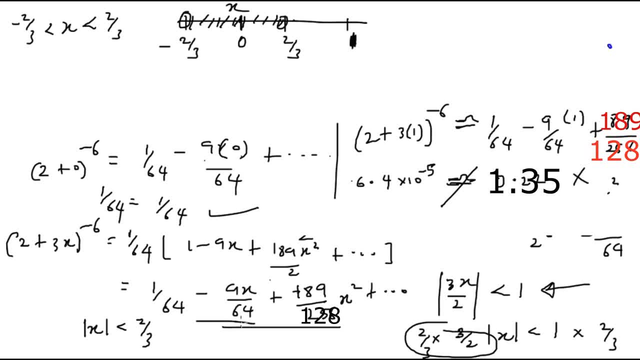 so it means that outside the region, the inequality, values of the inequality, will not tally, it will not be equal to each other, it will not be correct. but inside the region the inequality will be valid and that's why this inequality, 2 plus 3x, raised to power minus 6, is correctly equal to this. 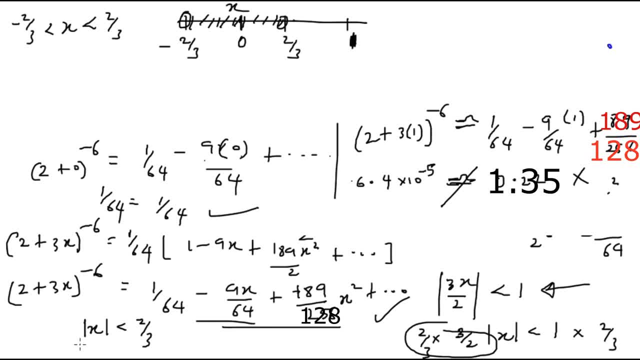 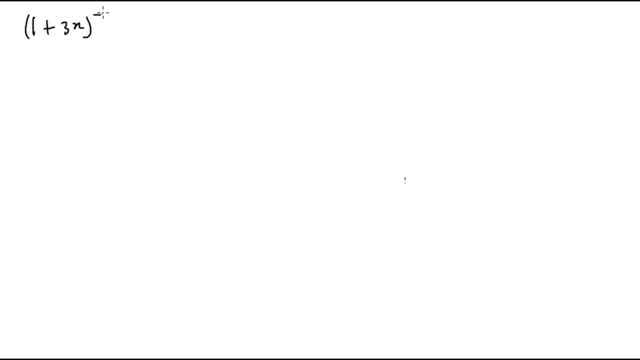 inequality, but only you understand, but only when the absolute value of x is less than 2 over 3.. so that's it about binomial expansion for negative integer. now let's solve one more exercise of 1 plus 3x, raised to power minus 2. okay, so it's. it has the form already, you don't need to go ahead. 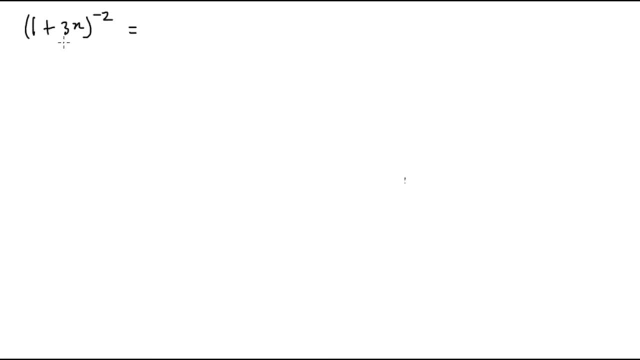 and start factorizing. you can factorize 3 out of it. if you factorize 3 out of it, then you will have 3 raised to power minus 2, 1 over 3 plus x, which is not the form. the form has to be 1 plus a particular. 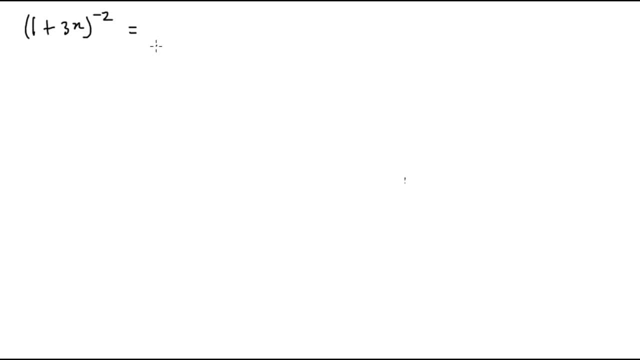 x. okay so, and you can factorize 3x out of it. if you factorize 3x out of it, you will have 3x 1 plus. you know, you have 1 upon 3x plus 1 and that's raised to power minus 2, eventually your. 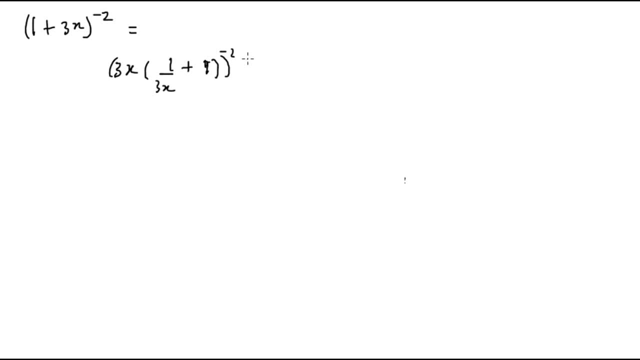 answer will be wrong. okay, because the range of values. it will not be valid if it tells the and if it tells the answer you have in your range of values, it should not be valid. so you don't take out, you don't factorize x, you only factorize the constants. okay, so that you can have one plus okay. so 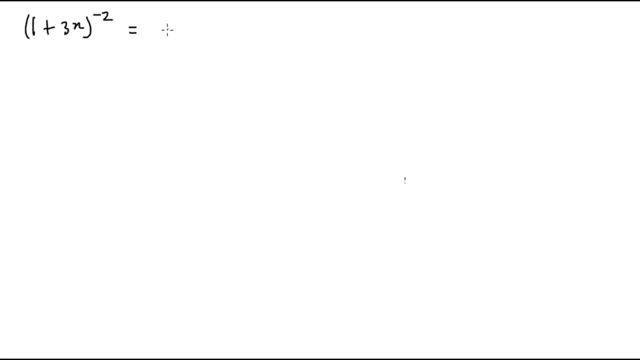 now it's already in the form because i have one, so i just need to continue to use the formula. so then that's one plus n. my n is negative, that's minus 2b. then my b is what is 3x is as simple as that. 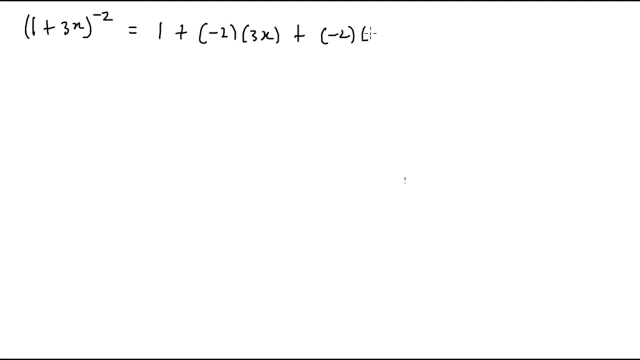 plus n again, which is minus 2. the next one is n minus 1, that's minus 2. minus 1, that's minus 3. okay, then i need to have b squared, that's 3x squared. don't forget: 3x squared is 9x squared, okay. 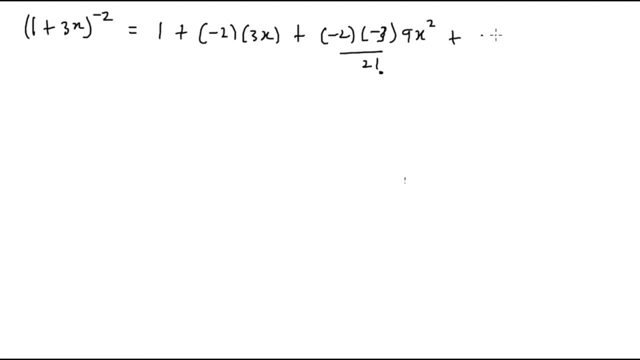 upon 2 factorial. i don't need to go too far, i can stop right here, all right. so if i want to go too far, i can just have it as the next one will be minus 2. that's my n. the next one will be minus 2. 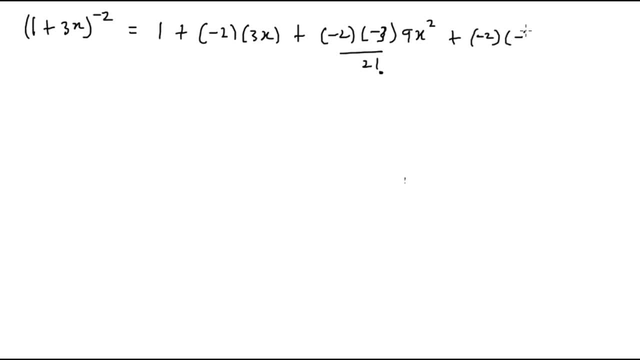 that's my n. the next one is n minus one. that's minus two minus one. that's minus three. the next one will be n minus two. that's minus two minus two. that's minus four. okay, this is n. this is n minus one. this is n minus two. so it's as simple as it does that n is negative. okay, so in at this. 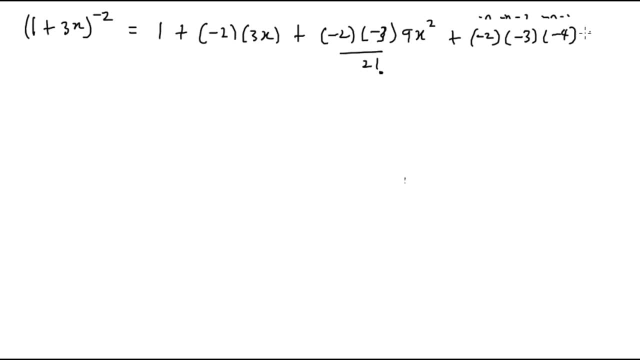 point. i will have three x cube, three cube and x cube, so three x cube, okay. cube raised to power three: okay. so if i want to avoid this, i can just have it as 27 x raised to power three, since three cube is the same thing as 27, okay. and then i'll have three factorial, so i just need to include. 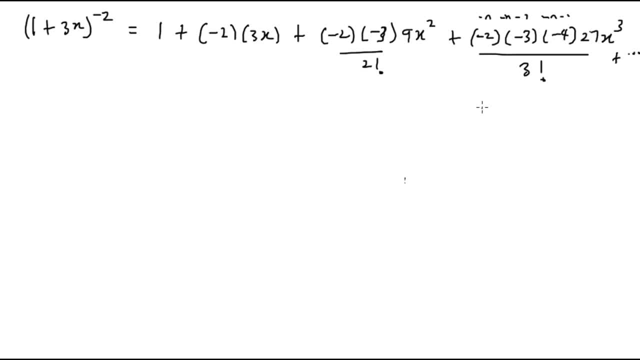 the dot dot dot because it's an infinite series. finally i'll have one then. minus six x, okay. minus six x plus 27 x squared plus dot dot dot- okay. so two. factorial is two minus minus. that's positive two. cancel out two, that's gone nine times three. 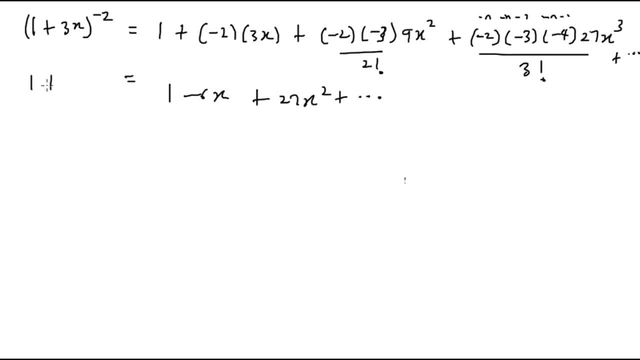 that's 27 x squared, so it's as simple as that. so i have one plus three x raised to power, minus two. but notice that that's this expansion is valid when absolute value of three x is less than one. i got it from this point, okay, so it's the same thing as three. absolute value of x is less than one is the. 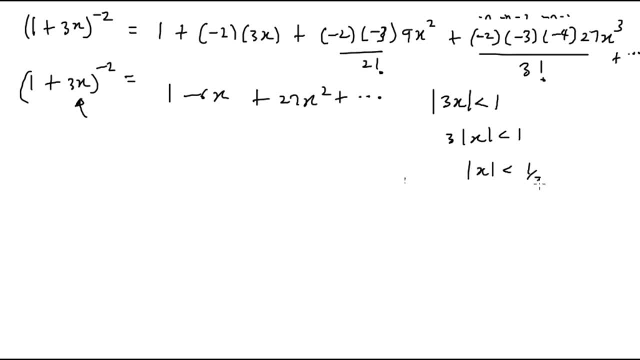 same thing as absolute value of x is less than one upon three, because i just need to divide both sides by three, divide both sides by three, so gone. so this is valid. so the implication of this is that the values of x will only range between minus one over three and one over three. that's the 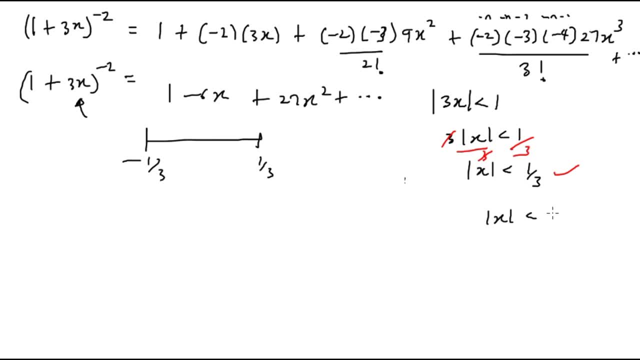 meaning of absolute value. if absolute value of x is less than a, that means x is less than a and x is greater than minus a. you can check my vg on absolute value inequality. so one over three is actually 0.33, so zero is between. so i can test zero, isn't it? so if i put zero right here, one raised to power minus two is still one. 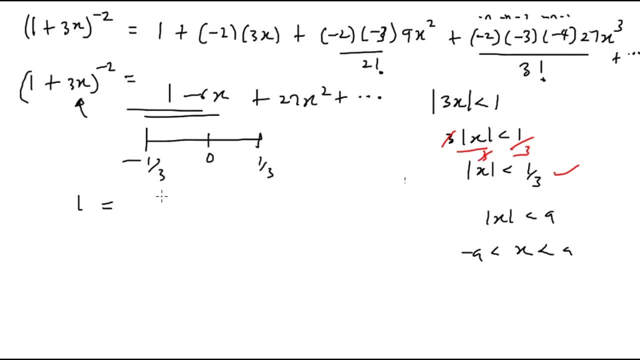 so i'm just testing. i'm done with the expansion. i just want to test so you can see if i substitute zero at the right hand side here. if zero is here, it becomes zero. zero is every other time we have zero, so that would be one. so it's valid, correct? but if i put a value outside the region, let's say 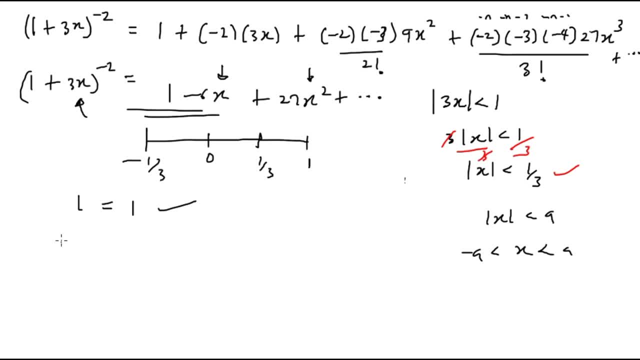 i put one. if i put one outside the region, i'll have one plus three. i will have one plus three raised to power minus two, equal to one minus six, into one plus twenty seven into one squared. okay. so that's one minus six plus twenty seven. one minus six plus twenty seven is twenty two, okay. 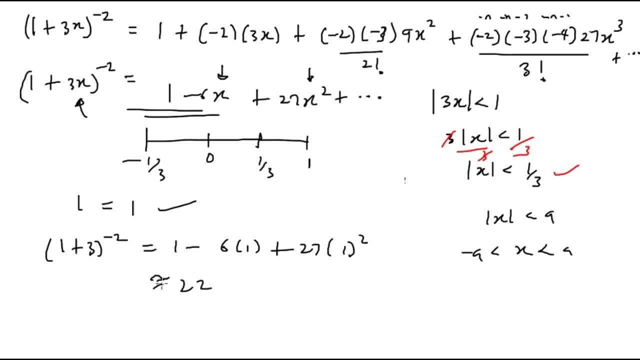 so at least i should have an approximate value of twenty two, even if it will not be equal to twenty 2 at least. so 1 plus 3, that's 4. so 4 raised to power minus 2 of course, that's 1 over 16. 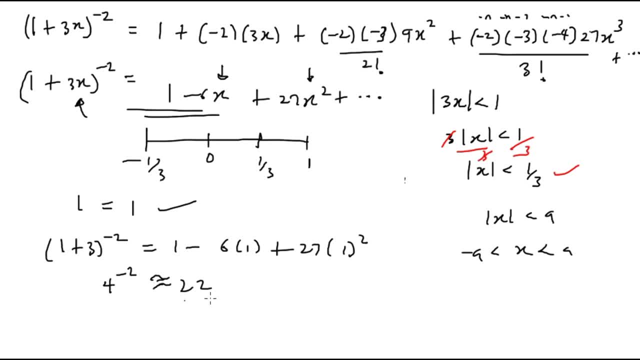 1 divided by 16 is 0.0. so which is not so, it is valid. this expansion is valid only when the absolute value of x is less than 1 over 3. let's say we have 1 minus x, raised to power minus 1. 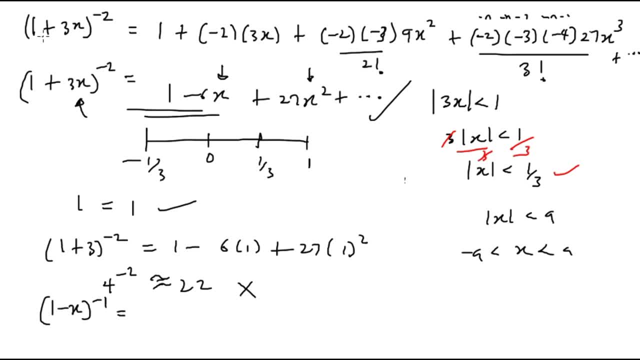 you see, this example is like this example: you don't need to factorize anything because you already have 1. so i can't say i want to factorize x out. just like i explained right here. you don't need to factorize 3x. so the expansion is also 1 plus nb. in this case, my n is minus 1 and my b is. 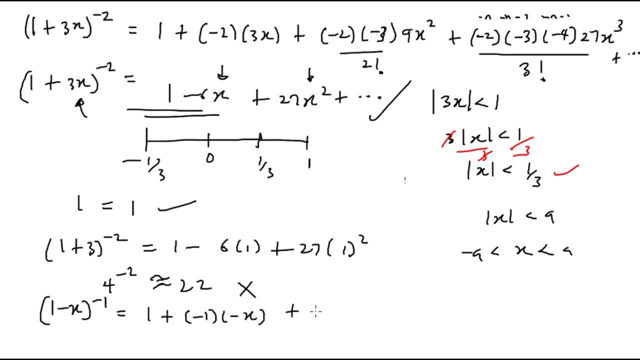 minus x. okay, plus n again, which is minus 1. so then n minus 1, that's minus 1. minus 1, that's minus 2. then b squared, that's minus x, squared upon 2, factorial plus dot dot dot. so if i simplify for that, we have 1 plus x. 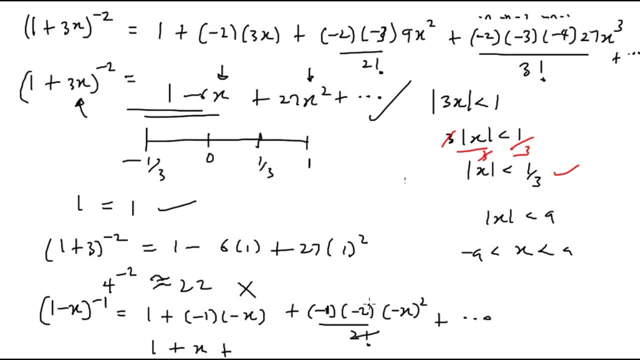 plus 2 factorial. we'll cancel out these two minus minus. that's positive. so i will have x squared plus dot dot dot. so it's as simple as that. so what i just need to do is to factorize minus 2 raised to power, minus x squared plus dot dot dot. so it's as simple as that. 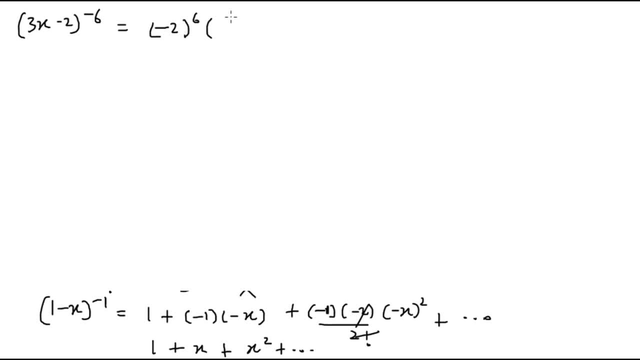 so that i will have 3x upon minus 2, then plus 1. i already factorized minus 2, so i just need to rewrite it as minus 2 raised to power 6, then 1 minus 3x upon 2 raised to power minus 6. okay, so i need to expand. 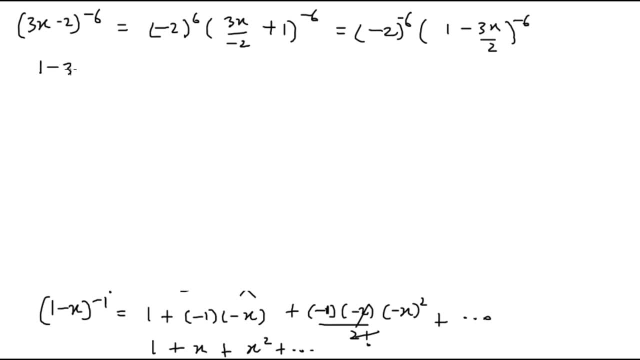 this: if i expand 1 minus 3x over 2, raised to power 6 minus 6, rather, i'll have 1 then plus minus 6 minus 3x upon 2, okay, that's 1 plus nb. you know the formula i'm using. this is the formula 1 plus b raised to power n, that's equal. 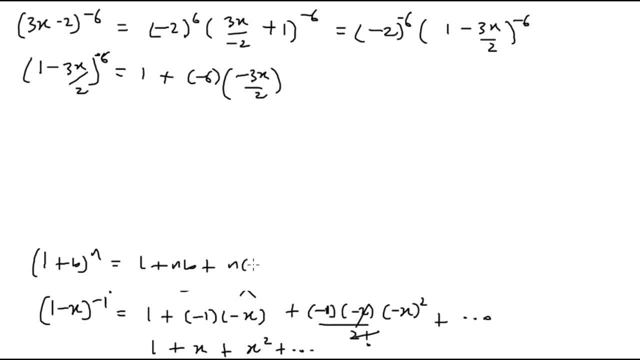 to 1 plus nb plus n into n minus 1, b squared upon 2 factorial. okay, so if this is n, the next one will follow by n minus 1. so the next one is n into n, into n minus 1, then i'll have n minus 2, then b squared upon 3 factorial. this is 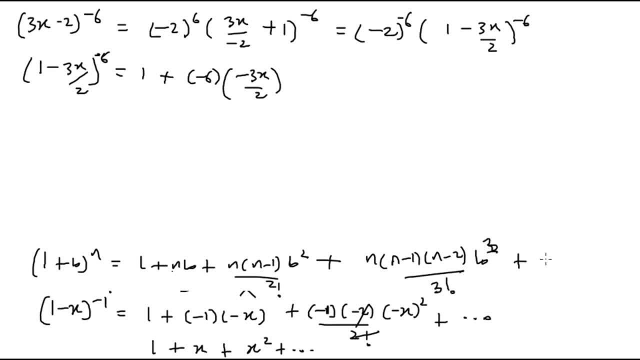 b cubed, because i already have b squared right, so it continues that way. so you just need to know the formula. so 1 plus nb plus n, again, that's minus 6, into n minus 1, that's minus 6 minus 1, that's minus 7, okay. and then i need to have minus 3 upon. 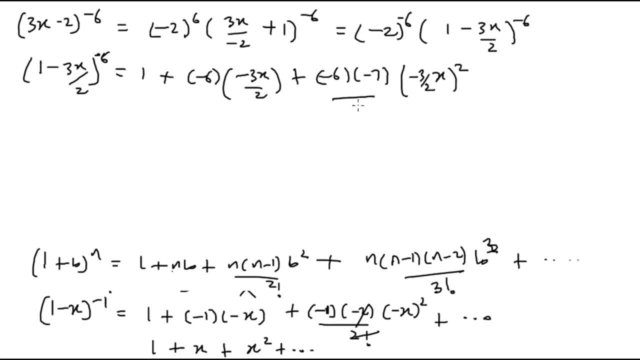 2, then x, then i have it squared upon 2 factorial- i don't need to go too far. okay, so it will be equal to 1 minus minus. that's positive. okay, so 2 in 6, that's 3. so i'll have 9x, okay, plus. 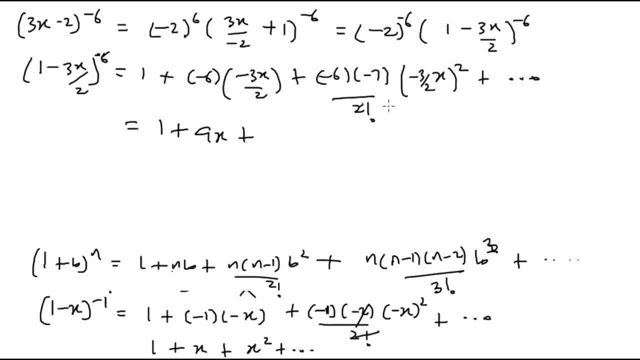 minus minus, that's positive. 2 here, 1. 2 in 6, that's 3. 7 times 3, that's 21. so i'll have minus inside the square. that's positive, isn't it? so it's still positive. does not affect the sign. so 7 times 3. 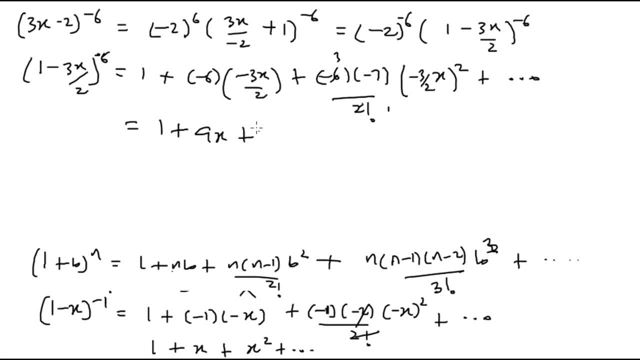 that's 21 multiplied by, so i'll have 189 upon 2, then x squared plus dot dot dot. so that's the expansion of 1 minus 3x over 2, raised to power 6. okay, so i can have it as, don't forget. 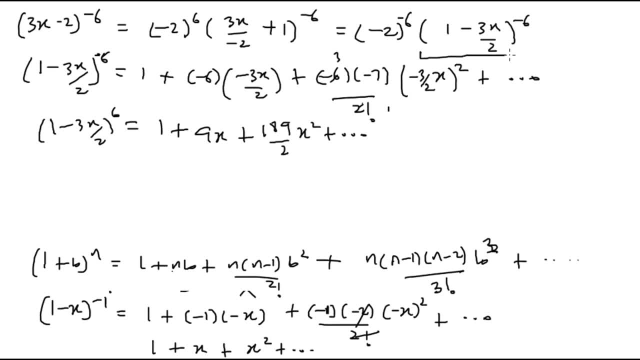 that this is just an expansion, an extension from this equation. so i'll have 3x minus 2 raised to power minus 6, which is equal to minus 2 raised to power minus 6, and then i have this binomial, so i can replace the binomial with its expansion, which is 1 plus 9x. 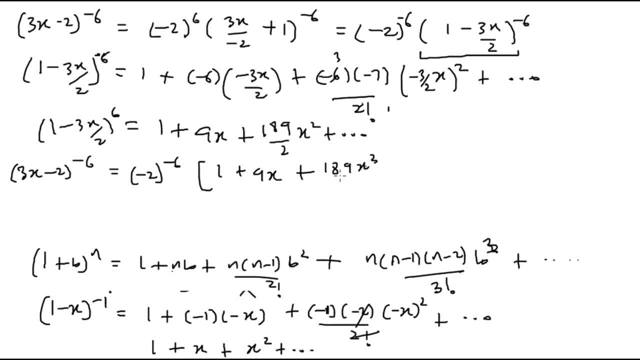 plus 189 x squared upon 2 plus dot dot dot is an infinite series, okay. it does not terminate. whenever n is negative, it does not terminate, okay, and that's why the condition is always very, very important. the condition, for instance, the condition for this expansion is this: the condition is always very important. the condition is minus 3x over 2. 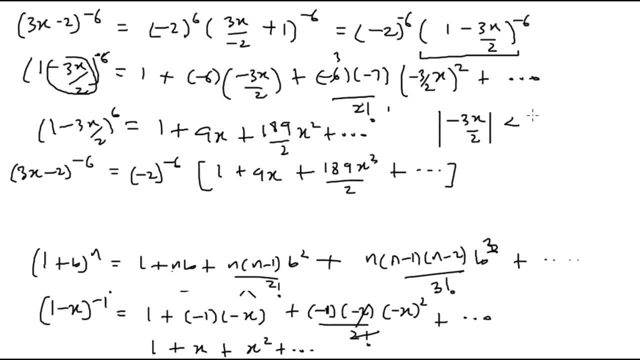 the absolute value of minus 3x over 2 has to be less than 1, which is the same thing as i told you will neglect the sign whenever we have absolute value. so that's 3 over 2x. so we can say that absolute value of x is less than 1. so it means that the absolute value of x is less than 2 over.